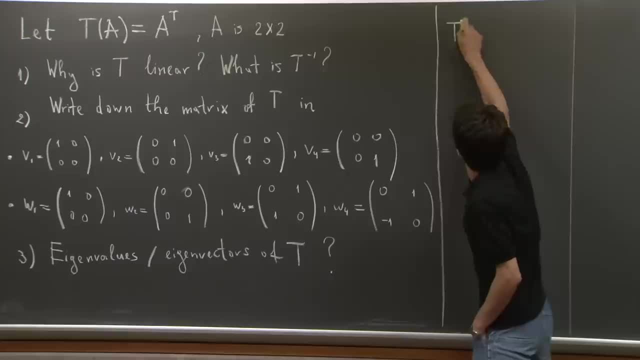 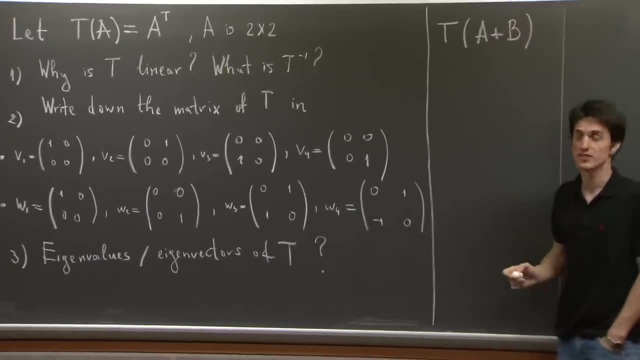 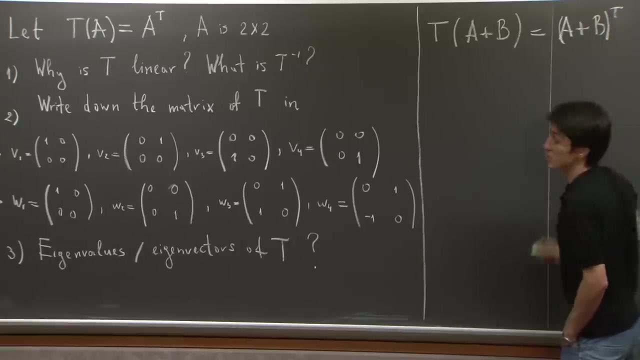 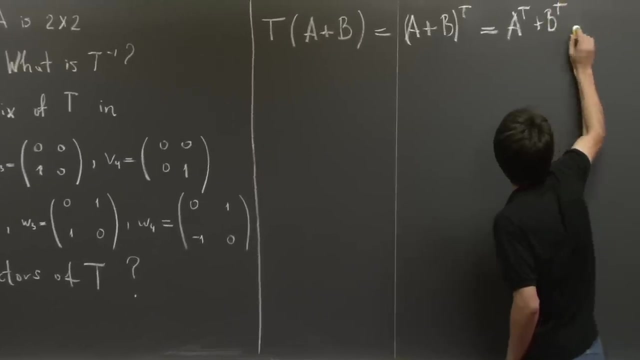 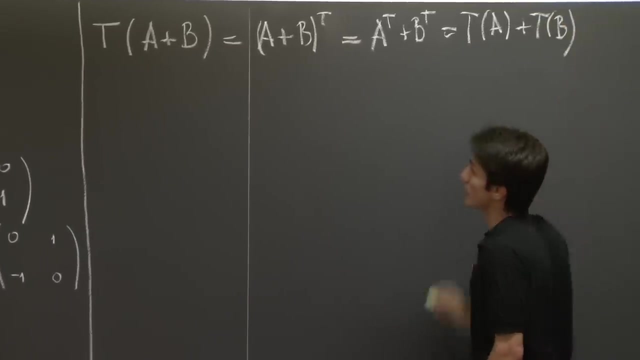 operator satisfies. Well, what happens when T acts on the sum of 2 matrices, A and B? So it produces the matrix, the transpose of A plus B. But we know that this is A transpose plus B transpose, And so this is exactly T A plus T B. 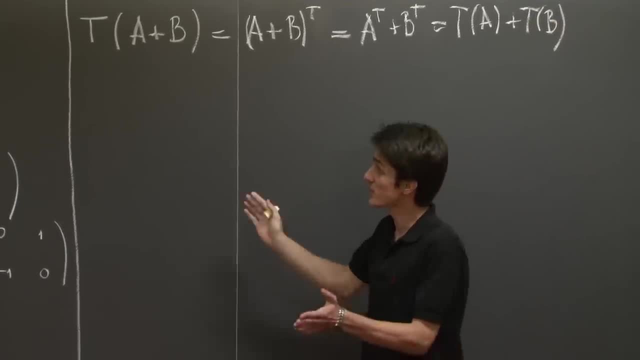 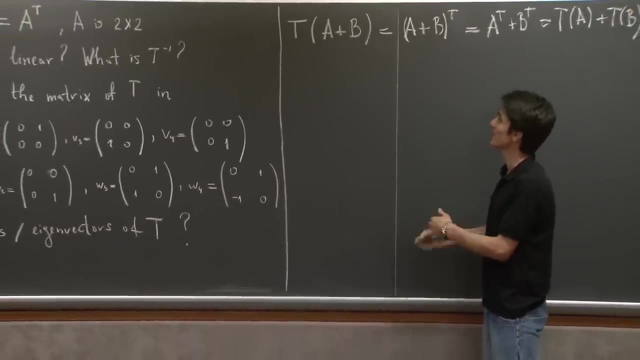 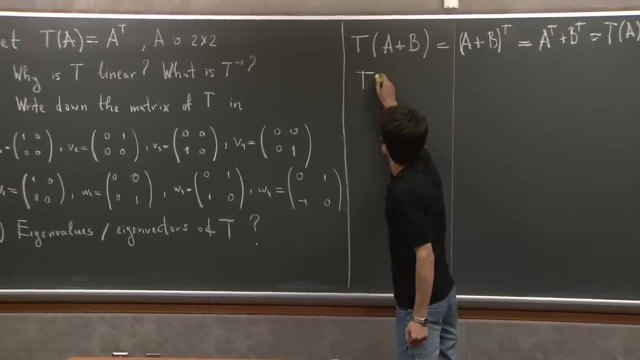 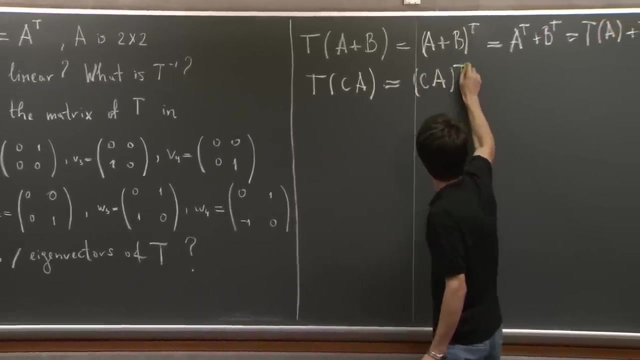 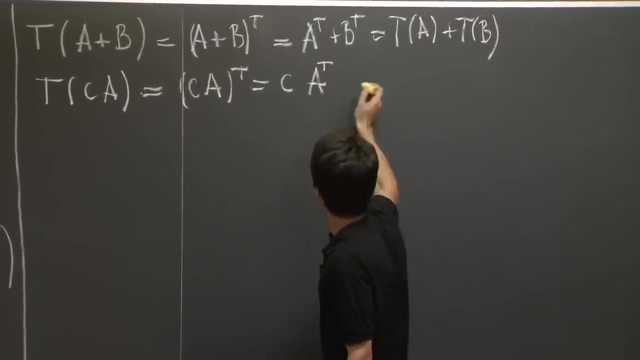 OK. so the transformation that we're analyzing takes the sum of two matrices into the sum of their transformations. OK. Similarly, it takes a multiple of a transformation into the multiple of the transformations. So it takes the matrix C times A to C times A transpose. 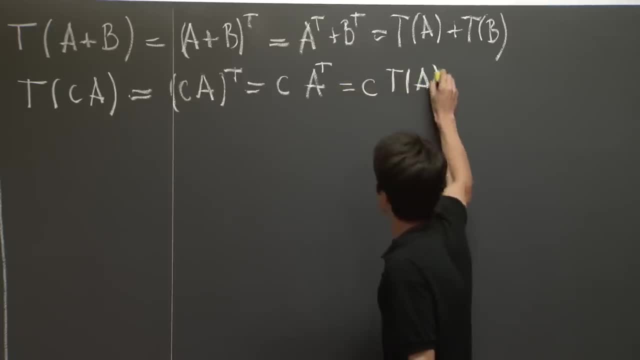 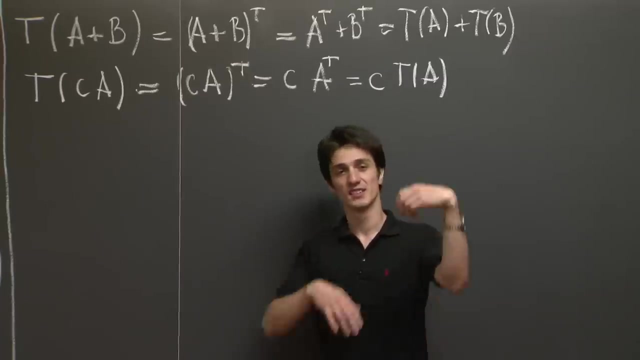 which is C, T of A. OK, so it is a linear operator. Now can we figure out what its inverse is? Well, what does the transpose do? It takes a column right and flips it into a row. So what happens if we apply the operation once again? 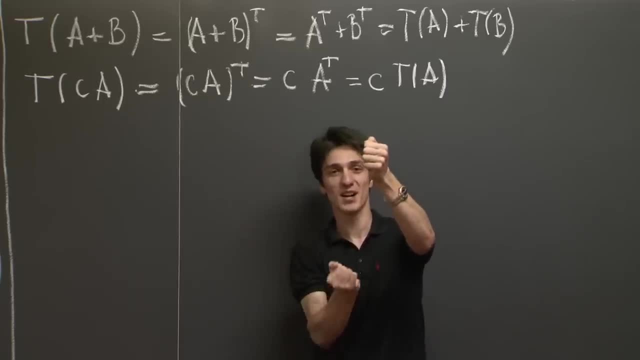 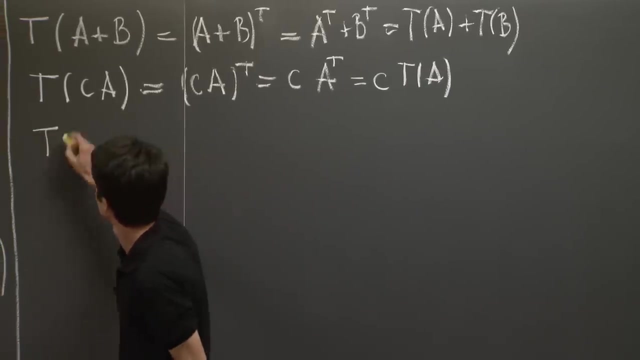 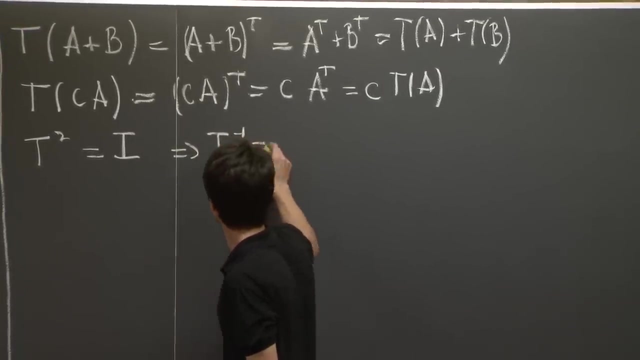 Well, it's going to take the row and turn it back down to the column, So, applying the transformation twice, we come back to the original situation. So therefore, T squared is the identity, And from this we infer that the inverse is the transformation itself. 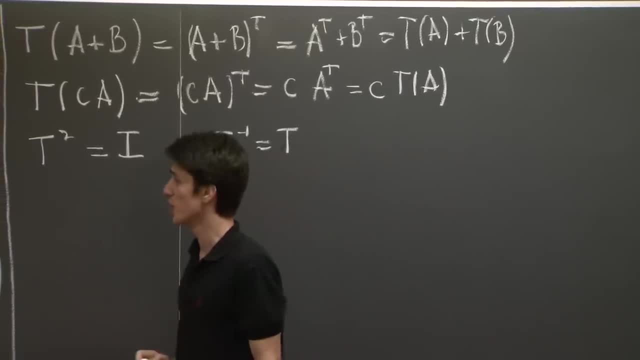 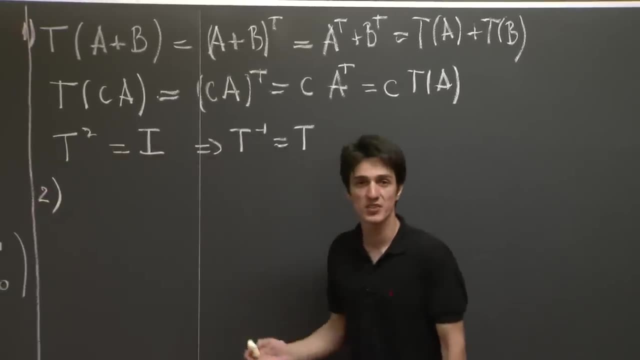 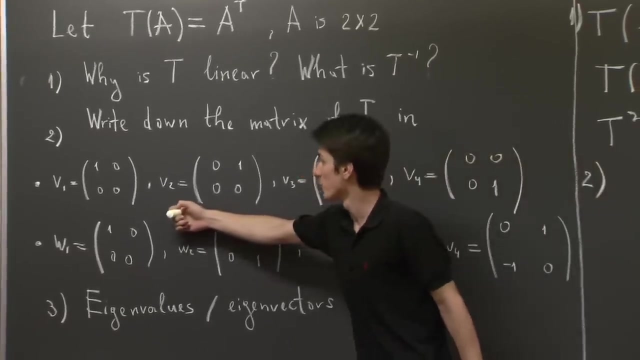 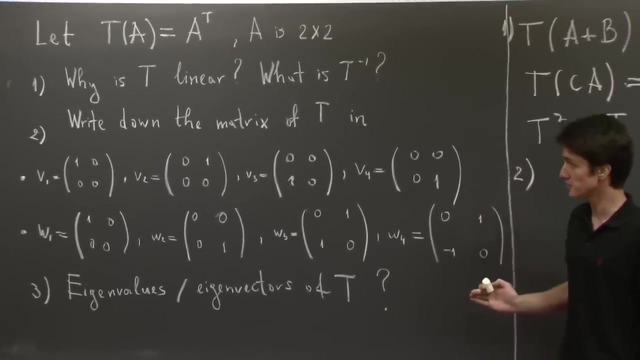 OK, now, this was part one. Part two: we'll compute the matrix of the linear transformation. We'll compute the matrix of the linear transformation in the following two bases. So the first basis is, in fact it is the standard basis for the space of 2 by 2 matrices. 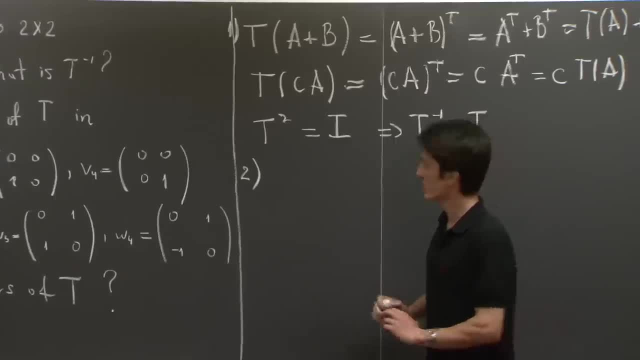 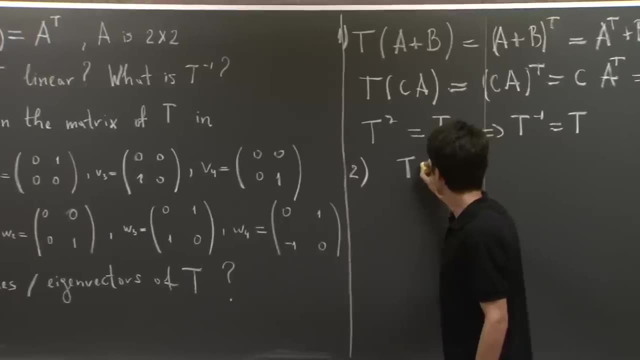 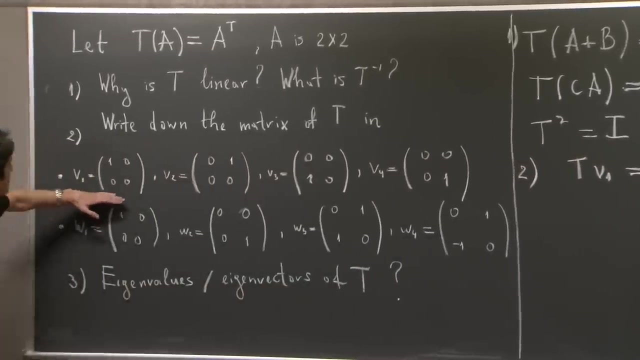 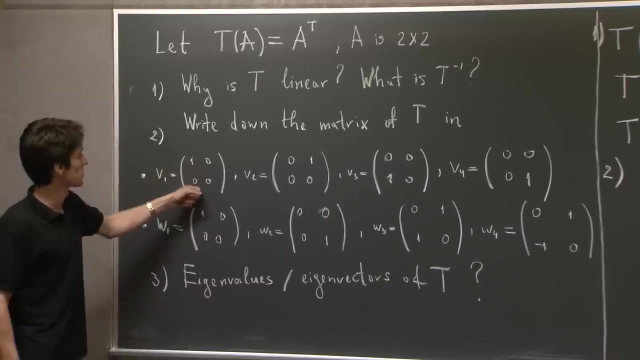 And the way we compute the matrix. we first compute what T does to each of the basis elements. OK, So T of V1.. OK, So it's here. So T takes the transpose of this matrix. But we see the transpose of 1, 0, 0, 0 is 1, 0, 0, 0.. 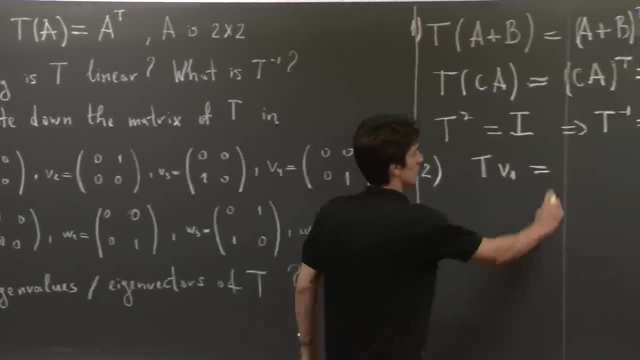 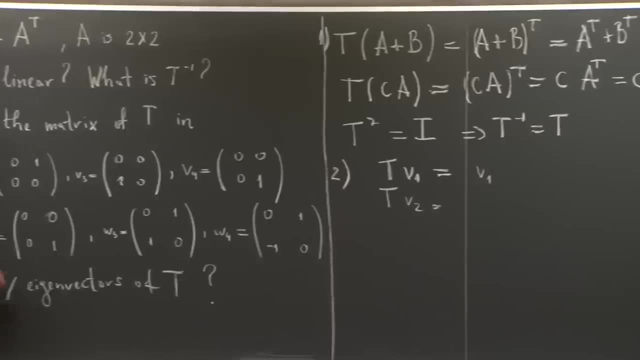 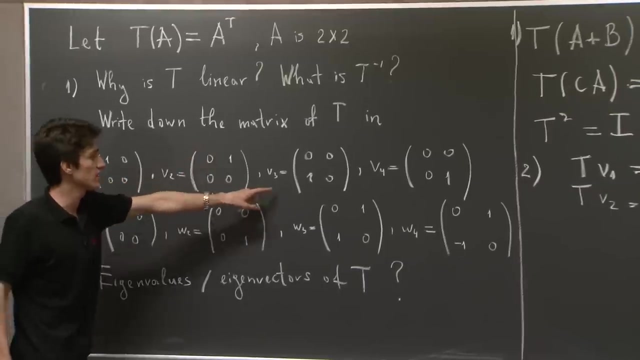 So it's a symmetric matrix. So T of V1 is V1.. What about T of V2?? Again, we come back here. So this one comes here, 0 comes here, And so we actually get V3, right. 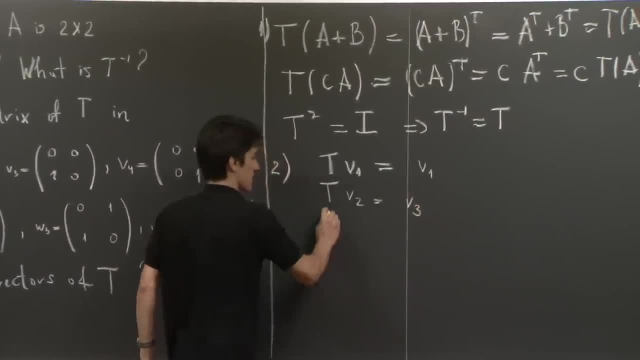 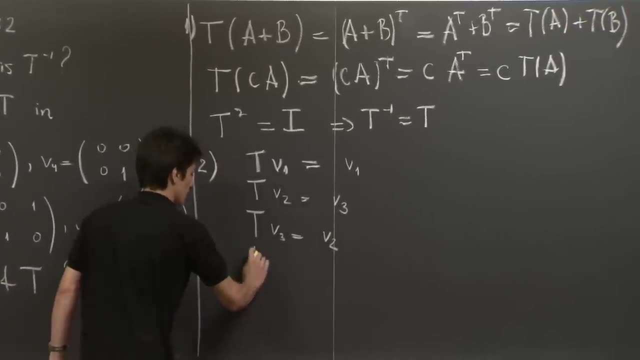 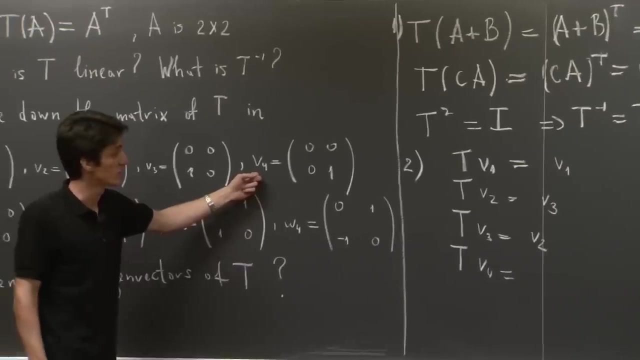 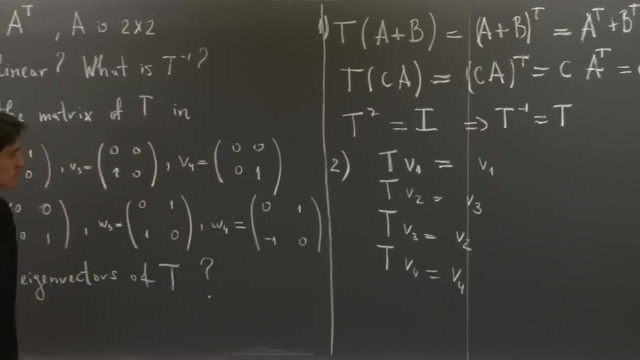 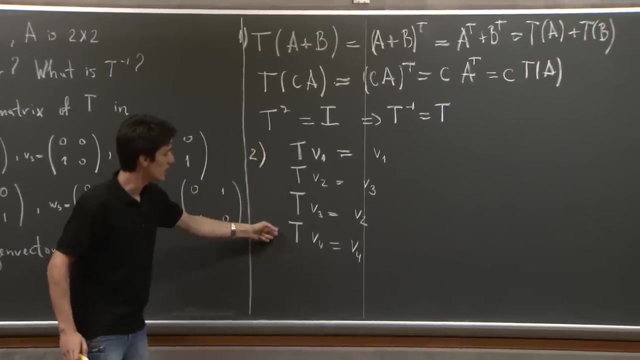 So T of V2 is V3.. Similarly, T of V3 is V2.. And finally, T of V4.. Well, V4 is a symmetric matrix as well, So the transpose doesn't change it. OK, So what we have now? we encode this into a matrix. 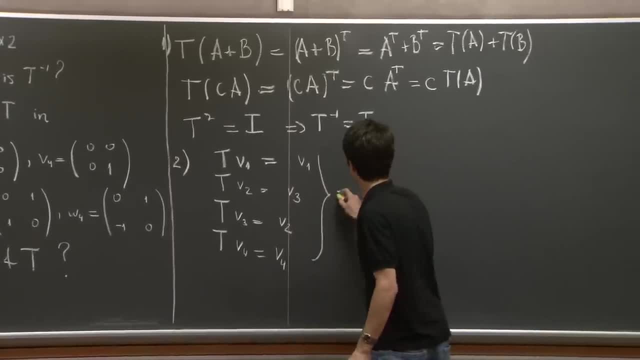 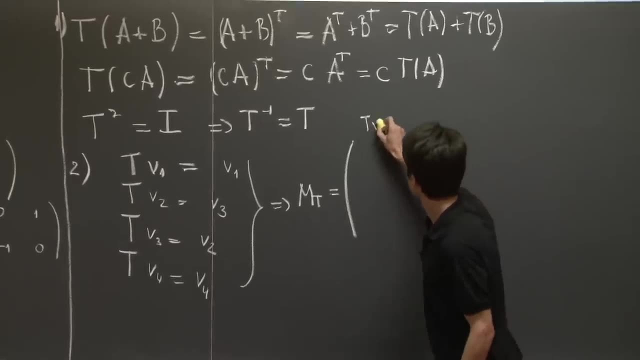 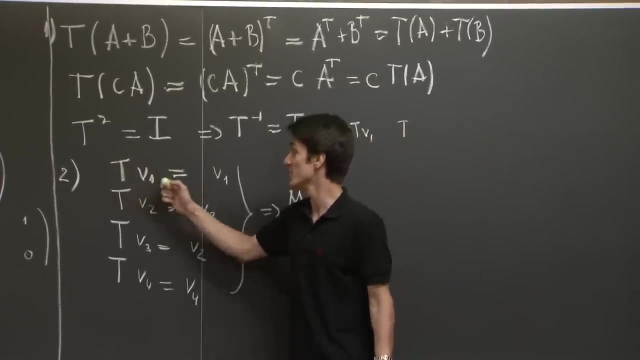 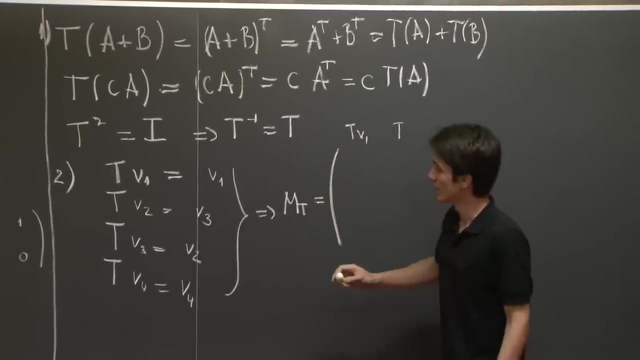 in the following way. Essentially, the first column will tell us how T of V1 is expressed as a linear combination of T of V1.. OK, OK, OK, OK. The basis element? Well, in this case it's just V1.. 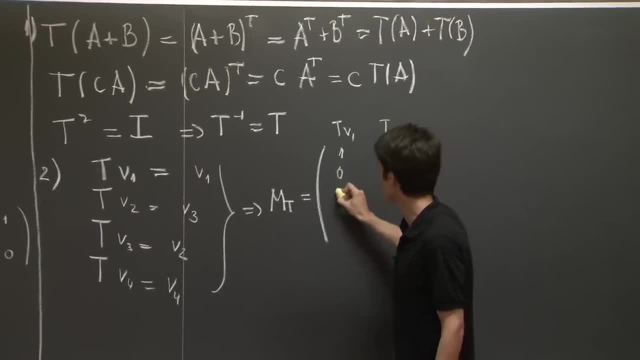 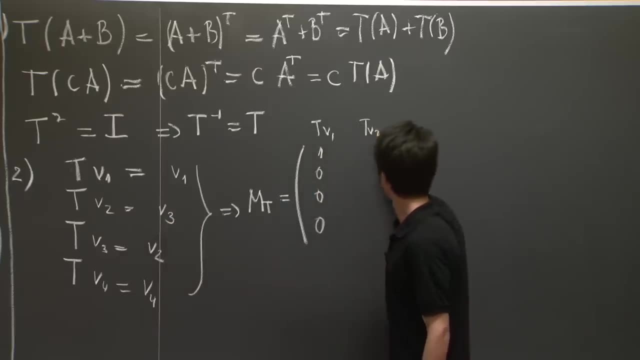 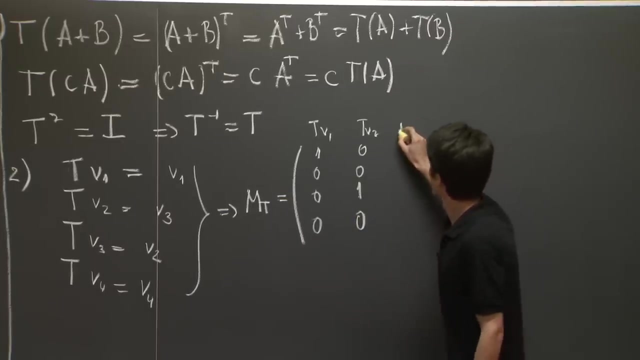 So it's going to be 1 times V1 plus 0, V2 plus 0, V3 plus 0, V4.. T of V2 is V3.. So we have 0, 0, 1, 0.. 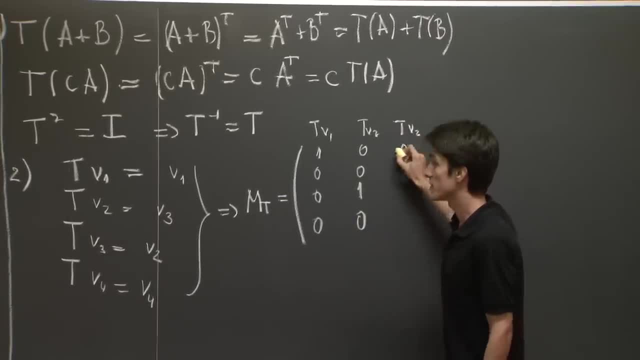 T of V3 is 0V1, 1V2, 0V3.. Watch- 1V2, 0, 2V3.. Rand- 0V4.. 0G, 0G, v3, 0- v4.. 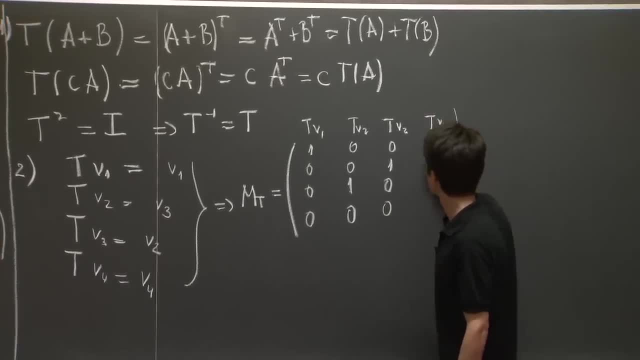 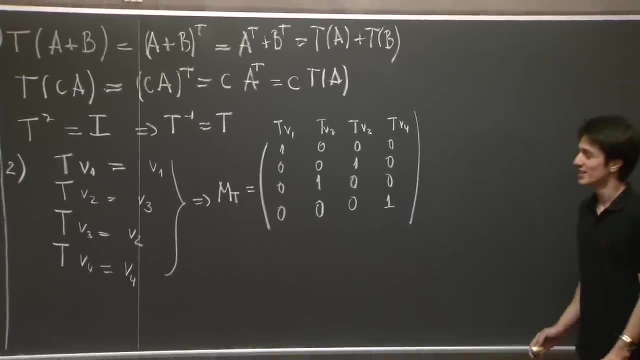 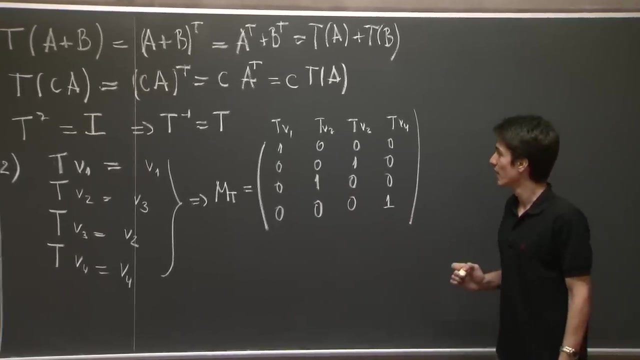 And T of v4 is 0 v1,, 0 v2, 0 v3 plus 1 v4.. OK, So we've written down the matrix of the linear transformation T in the standard basis And you can check that this is exactly what we want. 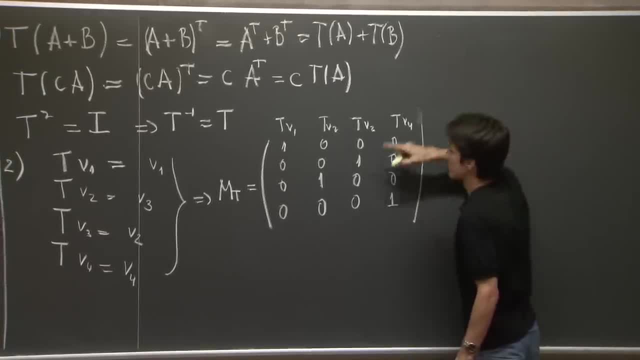 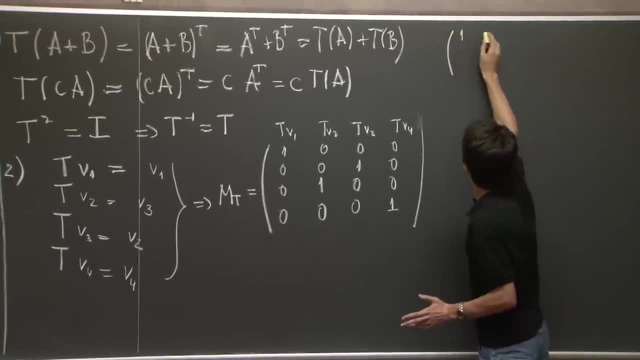 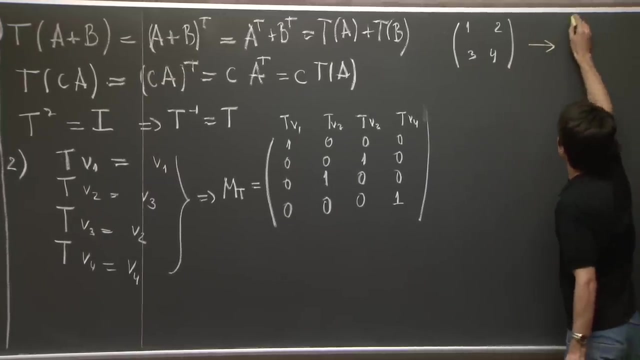 Say we can. yeah, let's see what this so yeah, Let's see what the representation of some matrix- say 1,, 2,, 3,, 4, in this standard basis is. It's the vector 1,, 2,, 3, 4.. 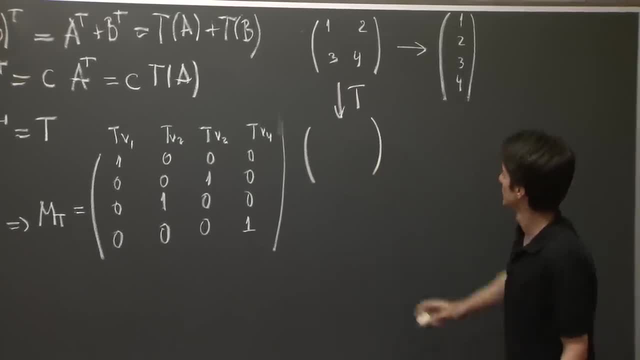 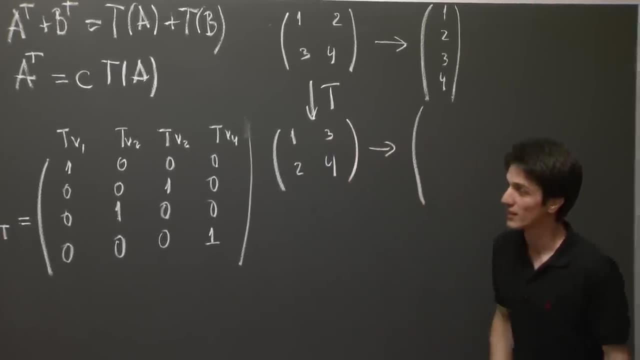 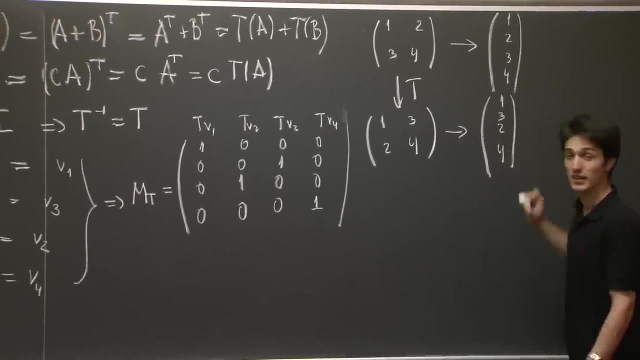 T takes this to its um Transpose: 1, 3, 2, 4.. So this in the basis is represented as 1, 3, 2, 4.. Right, And it's not hard to see that MT when. 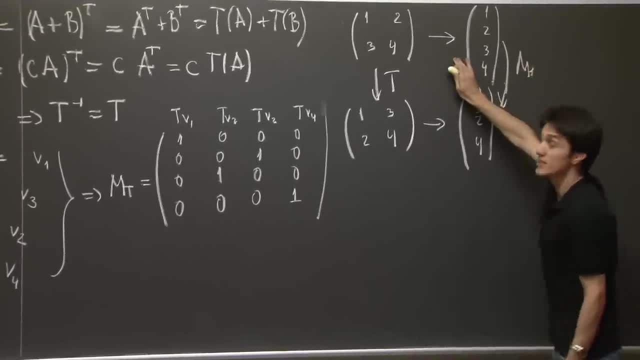 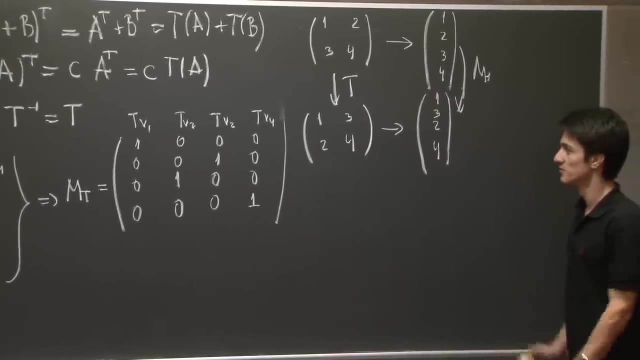 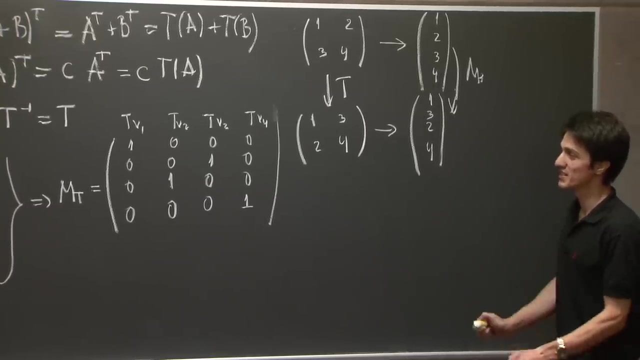 multiplies. when MT multiplies this vector, we get exactly this vector. OK, So we'll pause for a bit so that I erase the board, And we're going to return with the representation of T in the basis of w1,, w2,, w3, and w4., 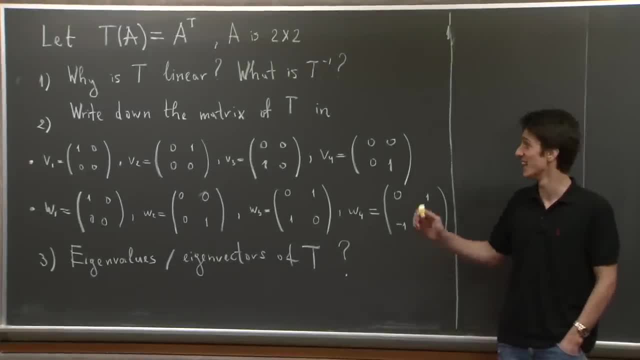 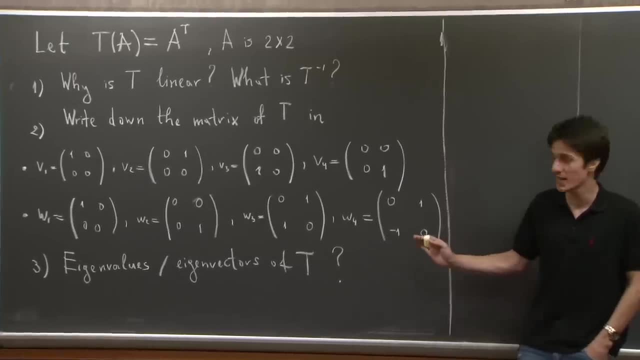 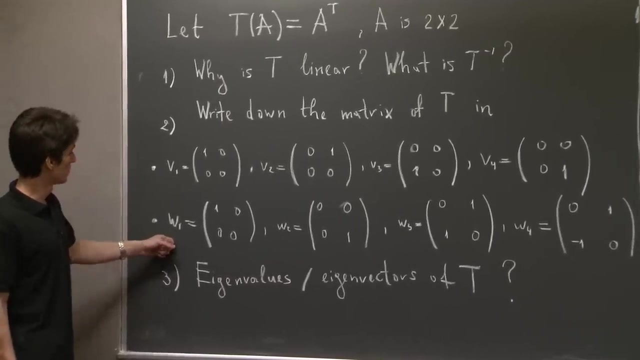 OK, So let's now compute the matrix of T in the basis w1,, w2,, w3, and w4.. We play the same game. We look at how T, T acts on each of the basis vectors, So T of w1.. 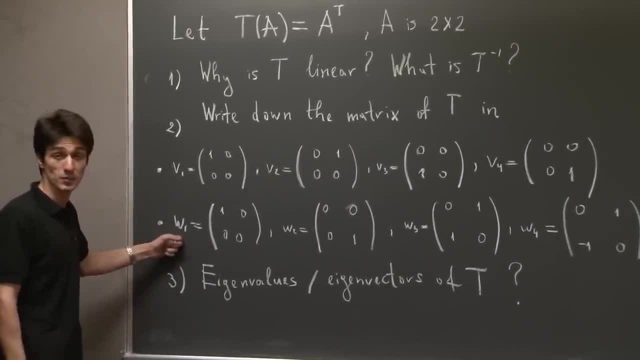 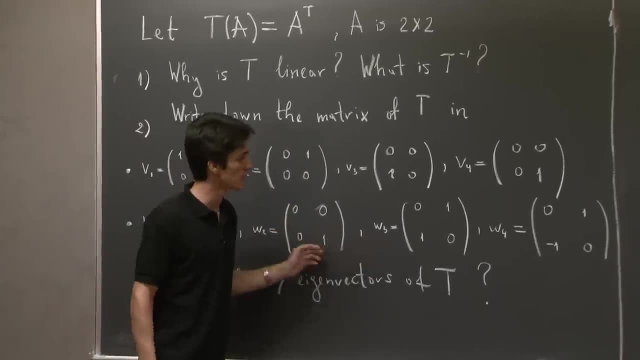 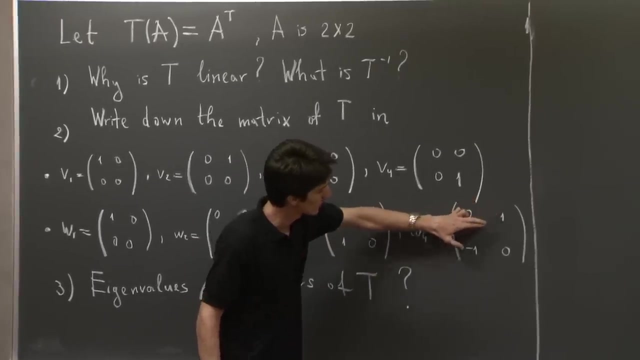 Well, w1 is a symmetric matrix, so T of w1 is w1.. Similarly with w2 and w3.. They're all symmetric. What about w4?? Well, we see that the 1 comes down here, The negative 1 comes up here. 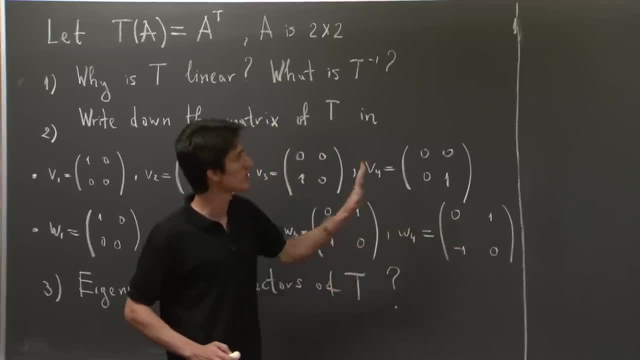 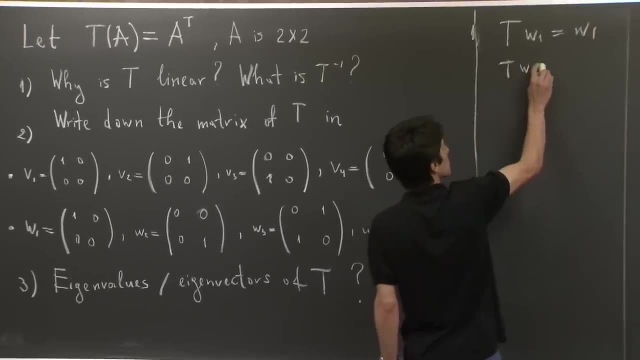 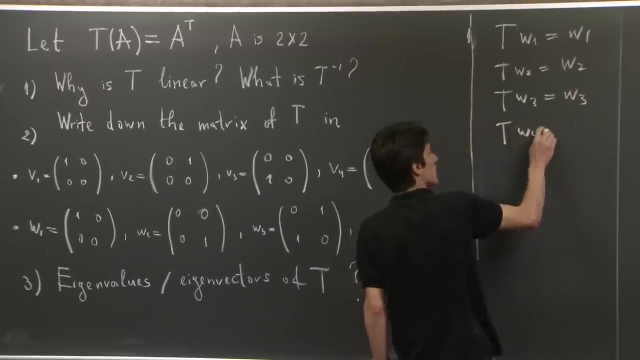 And in the end, we just get the negative of w4. So let me, Let me just write this out: We had T of w1 equal to w1, T of w2 equal to w2, T of w3 equal to w3, and T of w4 was negative of w4.